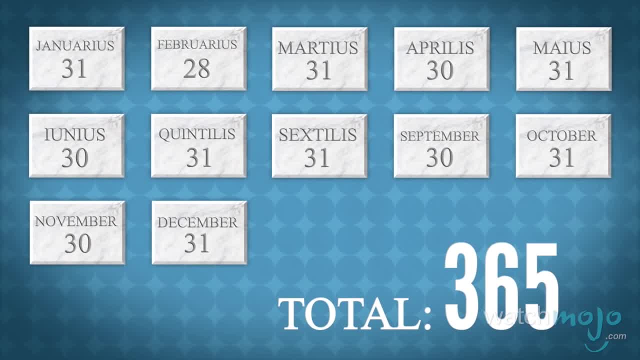 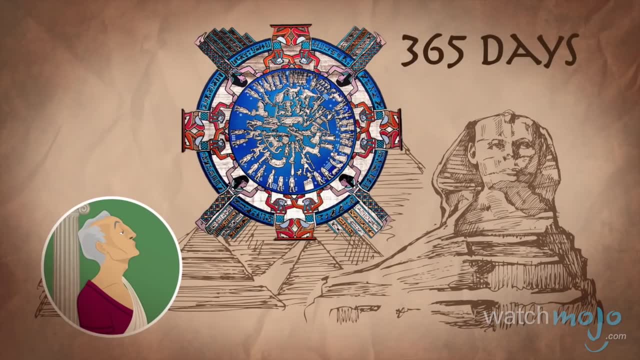 Rather than the 365 days we now observe, they added an extra 22 day month every two years. When the Julian calendar was introduced in 45 BC, it began the 365 day year, with an extra day added every fourth year at the end of February. 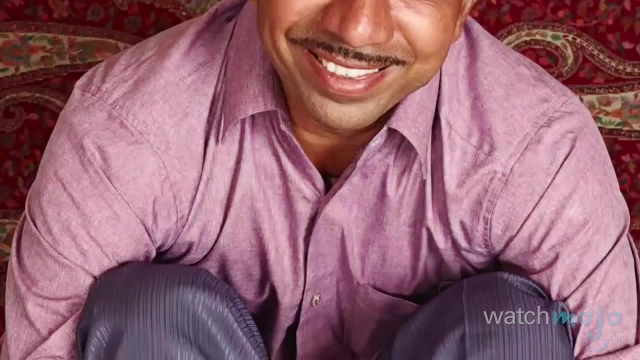 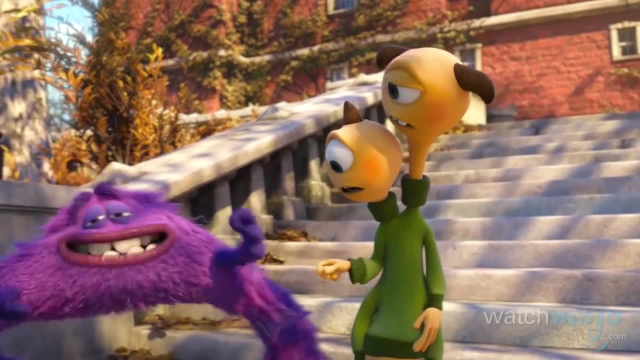 a practice we still uphold today. Leap year, motherfucker Number four, You have a higher chance of being born with an extra toe than you do of being born on February 29th. I have an extra toe- Not with me, of course. So the chances of being born on February 29th are 1 in 1,461.. So if my math is any good, there are roughly 187,000 people in America and around 4.5 million people around the world who were born on a leap day. 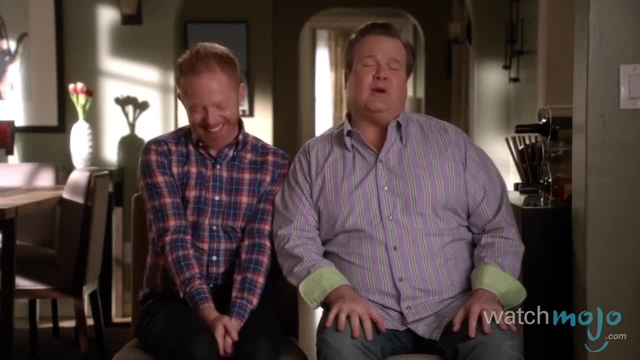 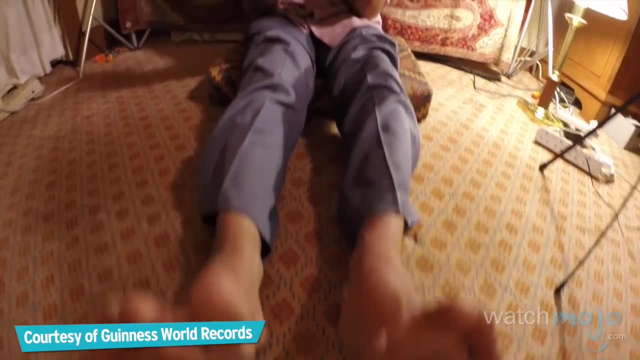 I'm 10!, 40!. I was born February 29th and there have been 10 of those in my lifetime. therefore, I'm 10!. Now, polydactylism is the condition where an individual is born with an extra finger or toe. 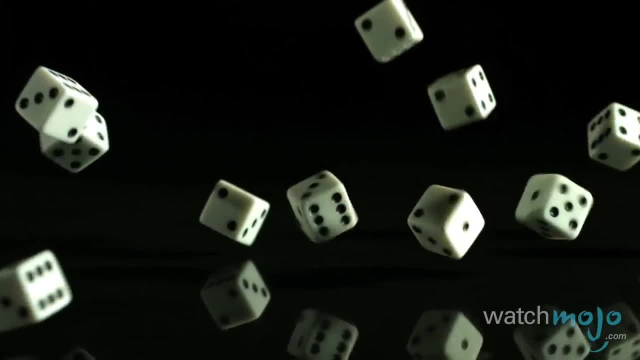 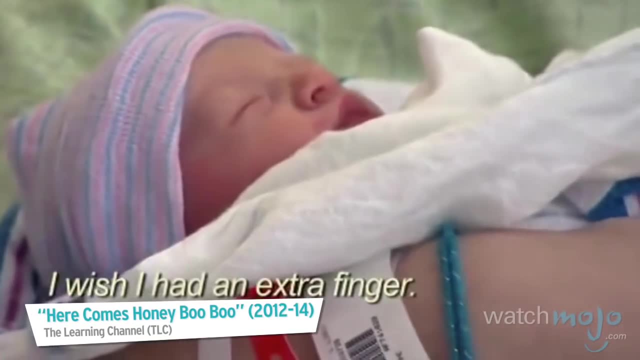 The chances of being born this way are around 1 in 500, meaning that you have a much better chance of being born with an extra finger than you do of being born on a leap day. I wish I had an extra finger, then I can grab my cheese balls. 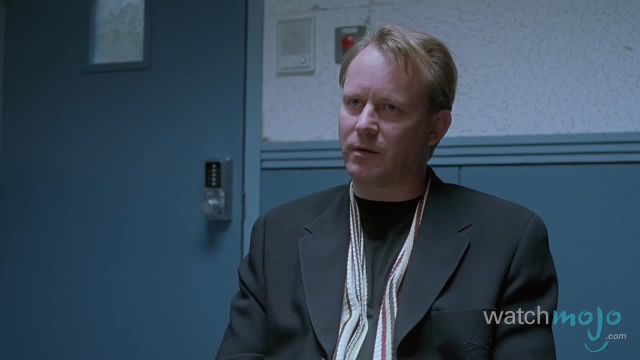 If anyone could work out the odds of being born with an extra digit on February 29th. you're better at math than I am Alright, I'll do the math, but I'm not gonna meet with any fucking therapist. Number three: 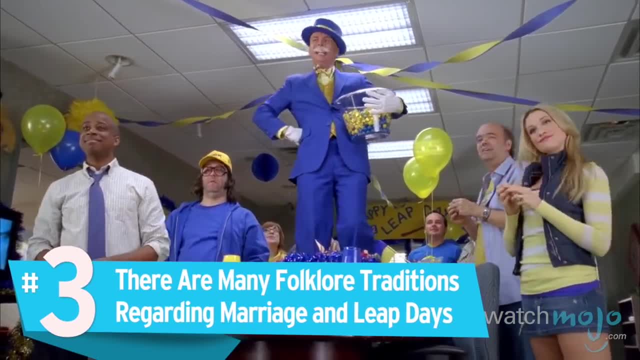 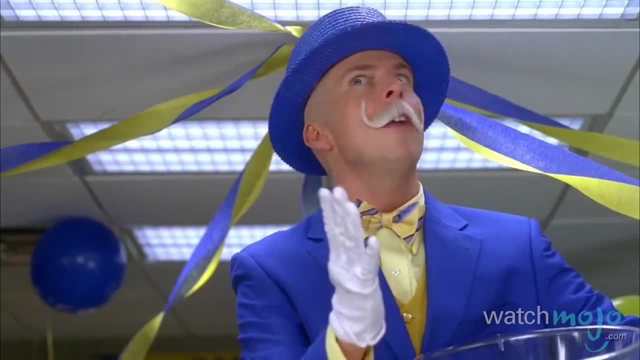 There are many folklore traditions regarding marriage and leap days, and we're not even referring to Leap Day, William. Did you not grow up with Leap Day, William? He lives in the Mariana Trench. he emerges every four years to trade children's tears for candy. 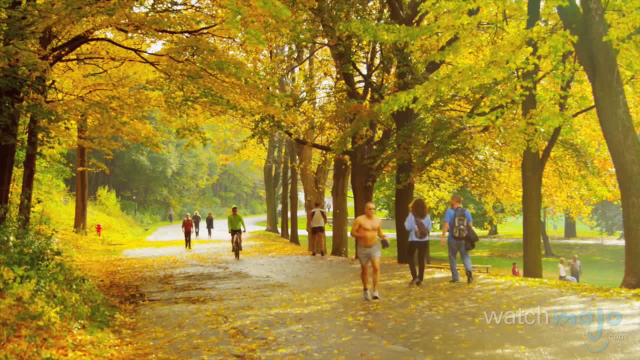 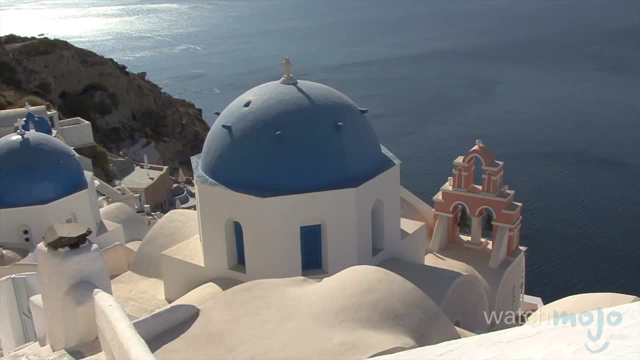 While a leap year may mean just another day for North Americans, leap days carry much more power around the world. In Greece, getting married during a leap year is said to be bad luck, and one in five couples will deliberately avoid planning their wedding for a leap year. 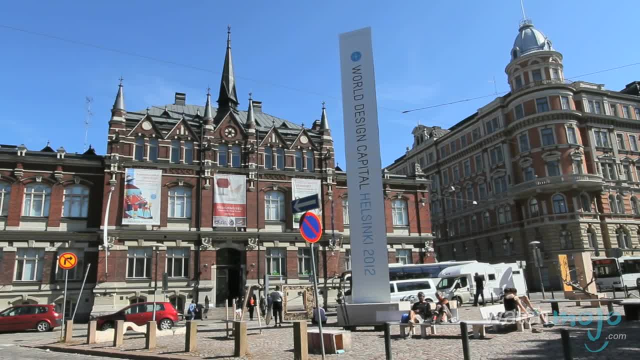 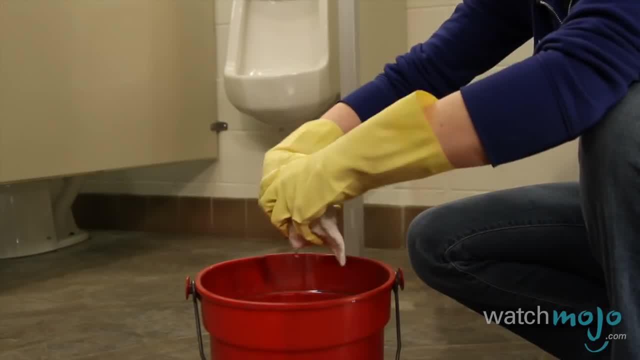 In Finland, Scotland and Ireland it is tradition for a woman to propose on a leap day, and if the man refuses, he has to give something in return. In Denmark, for instance, it was customary to give 12 pairs of gloves. 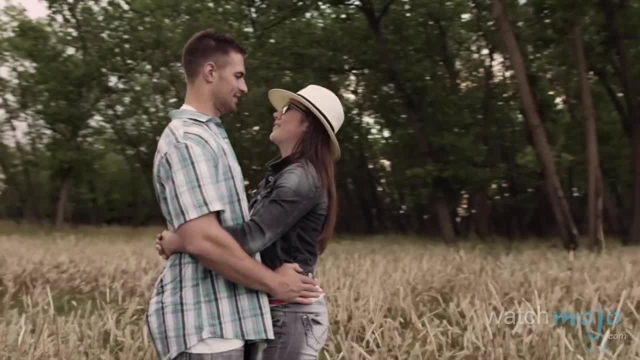 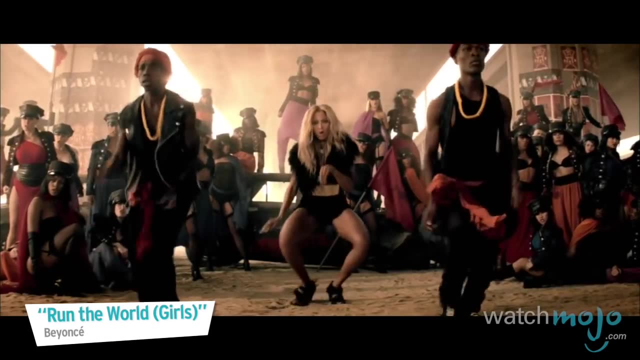 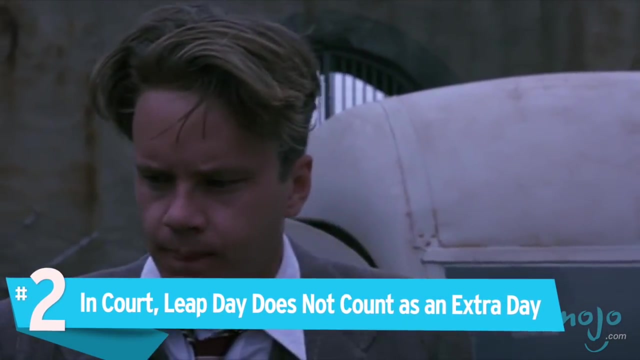 Critics have argued both for and against the tradition, with some arguing that it is outdated and maintains oppressive, restrictive gender roles, while others see it as empowering for women. Number two In court: leap day does not count as an extra day, But leap year is just that, isn't it? It's an extra day. Nevertheless, if you are sentenced to one year in prison during a leap year, you're going to the slammer for 366 days. That's not fair. In 2001,, an American woman tried to receive her dead ex-husband's social security benefits.